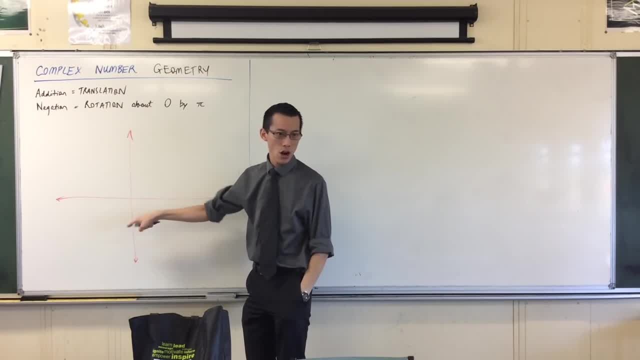 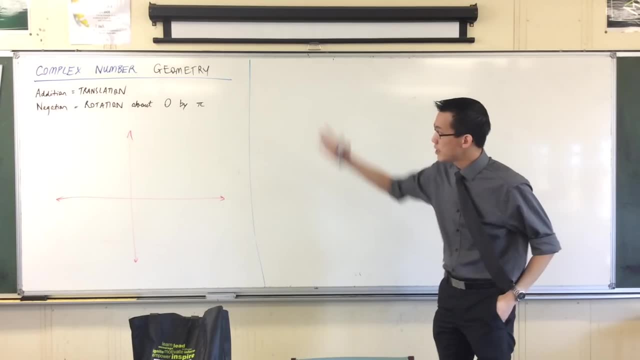 is that negation really means you rotate it around the origin by pi radians and that's what gets you from, say, the first quadrant around to the third. Now addition negation, which gave us subtraction. What operation is next? 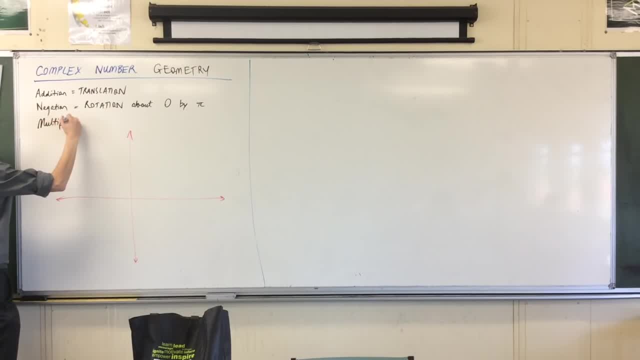 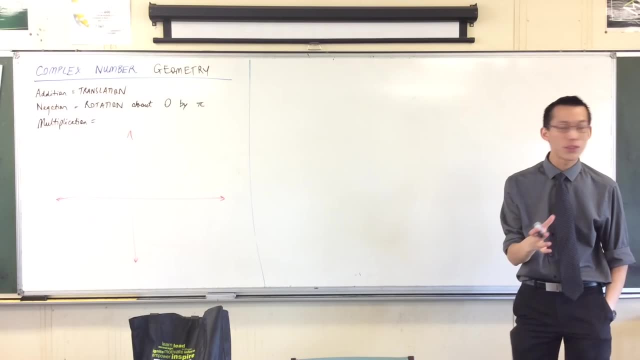 Multiplication. Okay, now to demonstrate multiplication for you, I'm going to abandon that Z1 and Z2 I gave you before. We can work with them, but this is starting to get a bit trickier, so I'm going to choose some very, very simple examples for you. 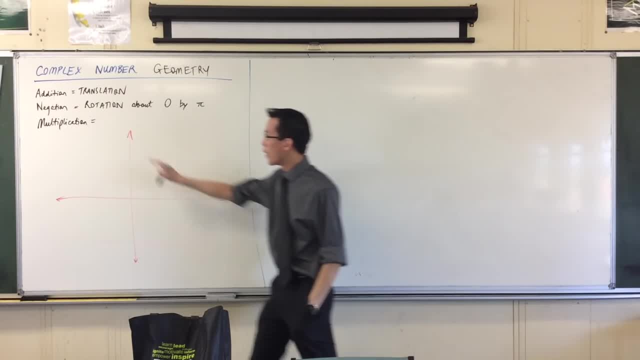 Okay. so for instance- and I'm going to just pop this up in the right-hand corner- we're going to fill this in like: what is multiplication? We'll do that after we've gone through this process. Let's just say Z1 is just the number 1.. 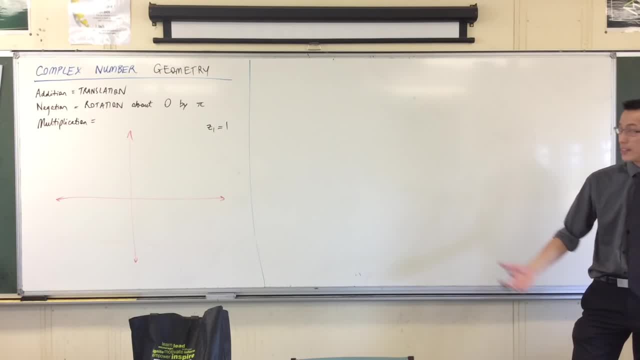 Now every real number that you know about actually is. Actually it is a complex number. It's just that it's got no imaginary component. okay, So 1 is still a complex number, It's just. I don't worry about the i's. 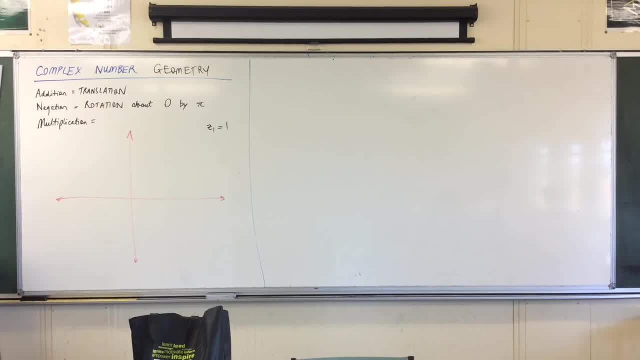 Where is Z1 on my diagram? It's going to be on the real axis, right, Because there's no imaginary part, okay, So I'm going to put him. I guess I'll place him like there, okay, That's Z1.. 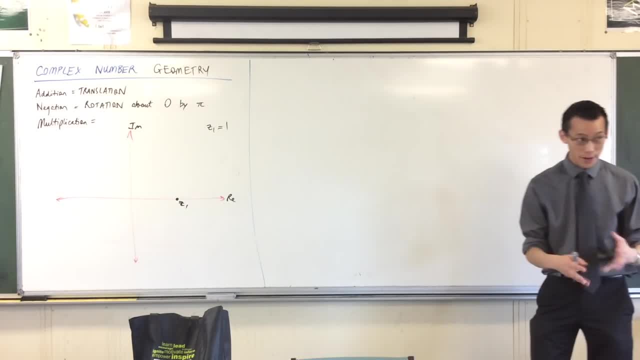 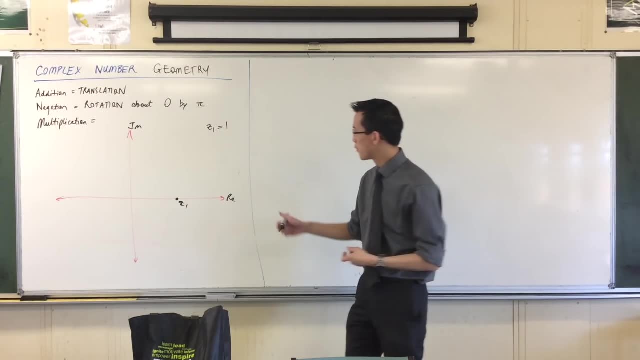 Now here's what I want to do. Like I said, I'm choosing very simple examples so I can see what's happening. I want to multiply by a number. Now, what's a nice, simple, complex number to choose For Z2,? I'm just going to go with i. 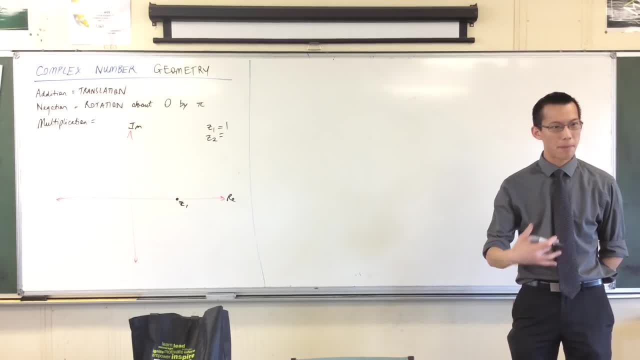 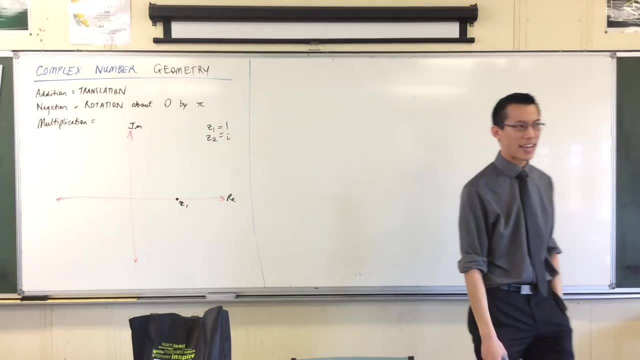 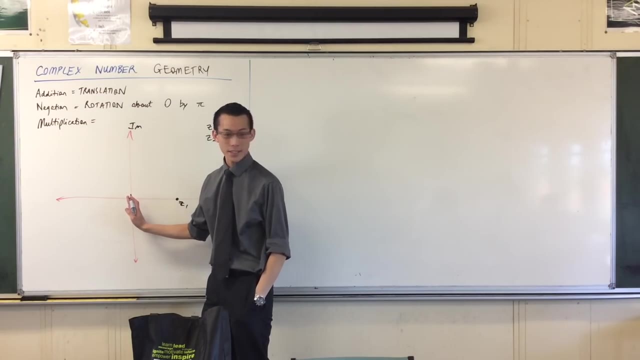 i is the quintessential complex number, right? So multiplying 1 by i just gives me i. Now where is i on my complex plane? okay, Being that i Z2, is purely imaginary, right? It belongs in line with 0 on the real axis, but it belongs up here. 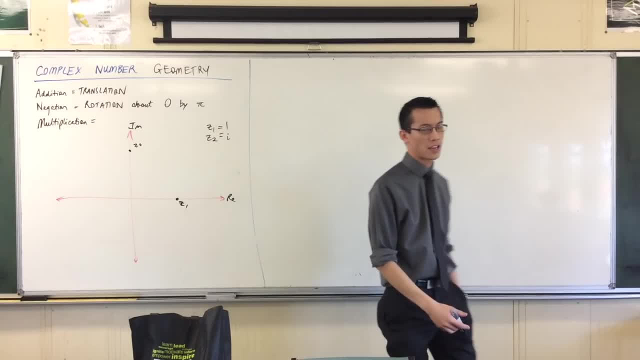 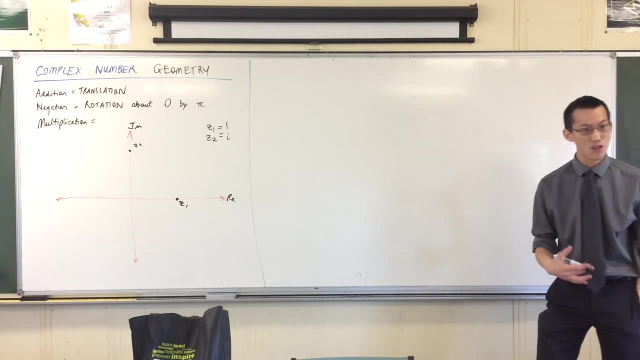 There's Z2, okay, Multiplying by i has taken me from there to there. Now, at the moment I don't know enough. You know how we're talking about series and sequences and you need three things for a pattern, right? 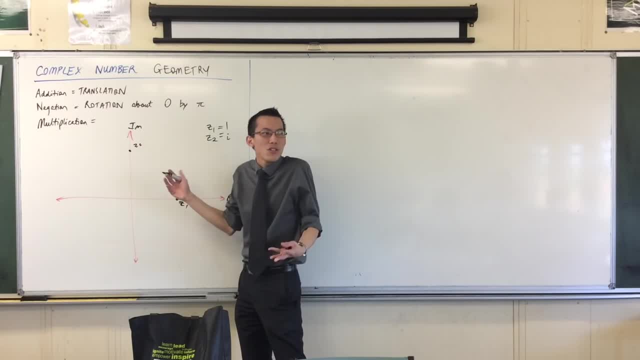 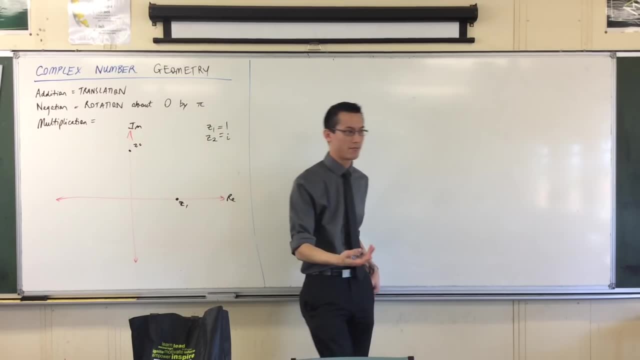 I've got two things right now, 1 and 2, but I don't know what's geometrically getting me from here to here. It could be translation, It could be reflection across the line. you know y equals x. if I wanted to. 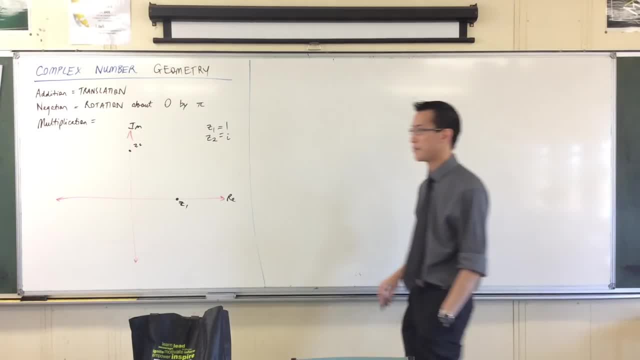 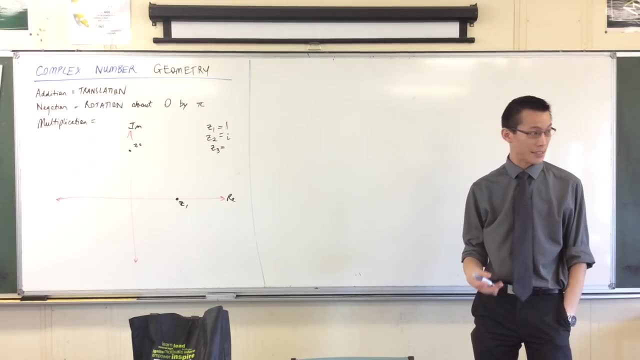 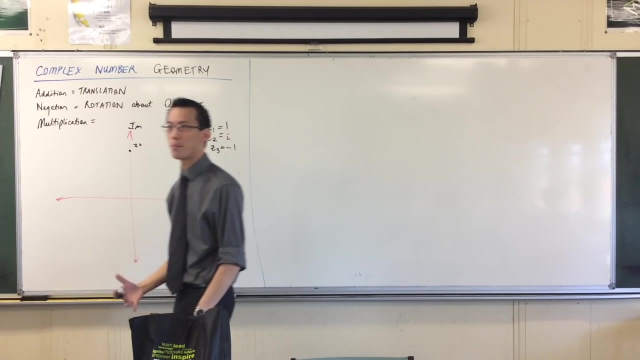 I don't know enough yet, So let's do it again, okay. Z3. When I multiply by i again I've got i squared now. but I know what i squared is: by definition: It's negative 1.. Where is negative 1 on my complex plane? 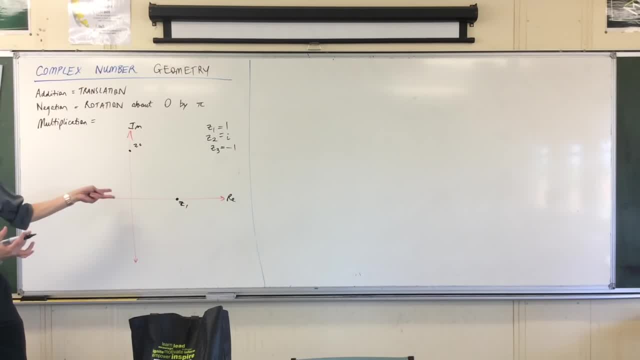 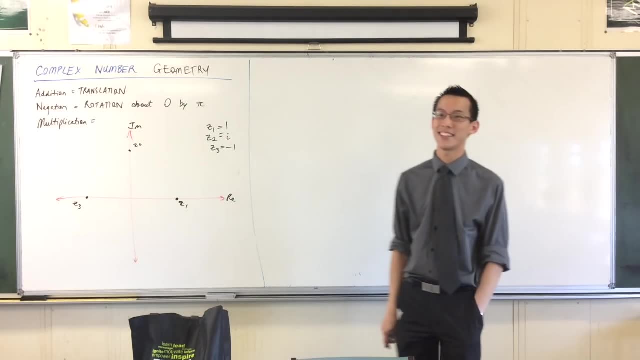 Negative 1 is completely real. It's purely real. okay, So I'm back on the real axis over here. okay, We're going to do it one more time to make it bleedingly obvious, If I multiply by i, one last time. 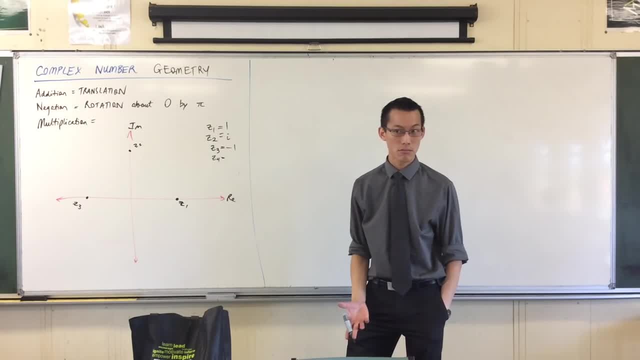 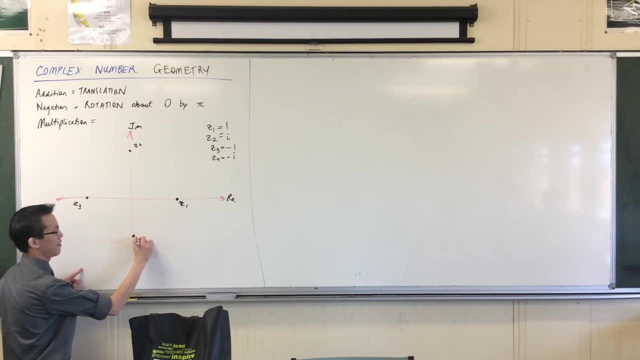 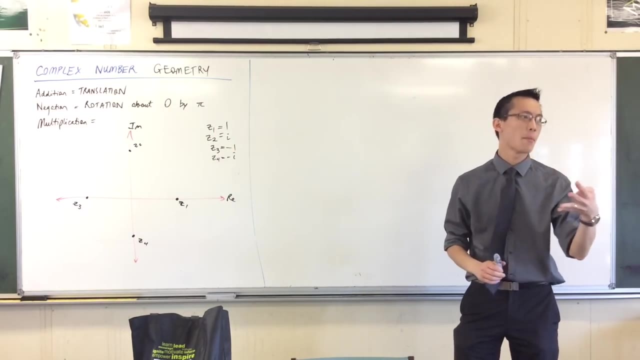 Z4 will be negative 1 times i, which is Negative i, Negative, i, And I won't ask it again This time. let's just spot this guy. He belongs down here on the negative imaginary axis. okay, Four times I have done the same operation, okay. 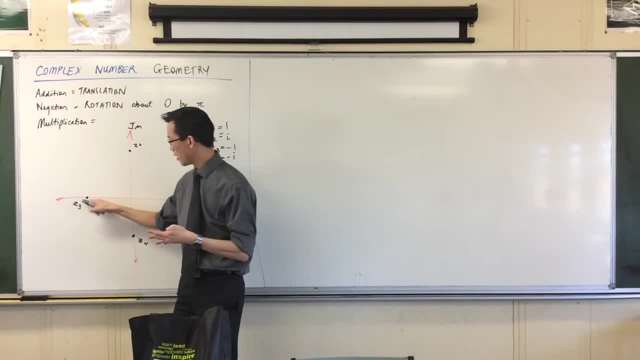 The first time I went from here to here. The second time I went from here to here, The third time: wait first, second. three times, of course, from 1 to 4.. Three times I've done this operation. 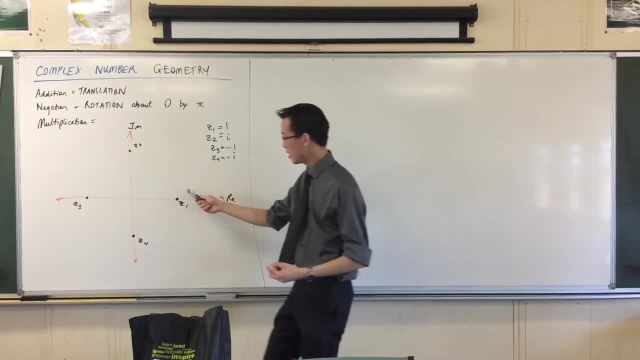 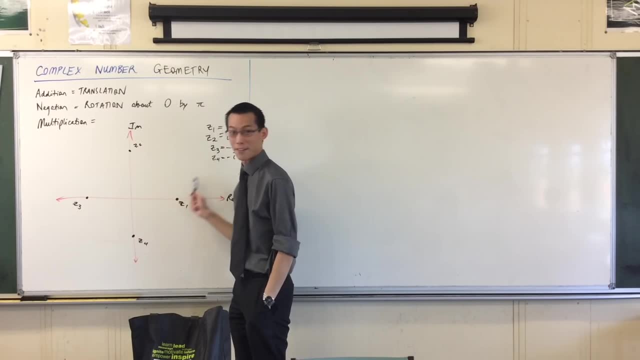 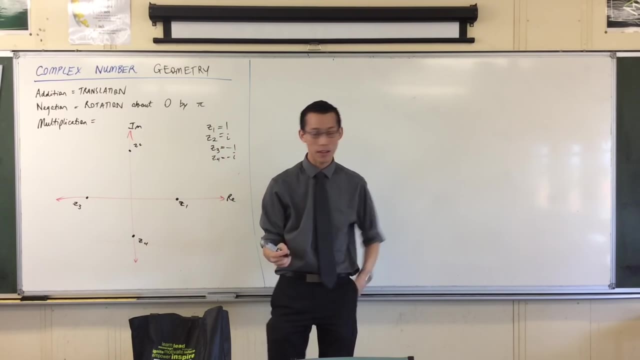 What is the geometric thing that gets me repeatedly from here to here, to here to here? And you can see, even in the way that I've drawn, like moving my hand right, I am clearly rotating around the origin. Do you see that? Okay, 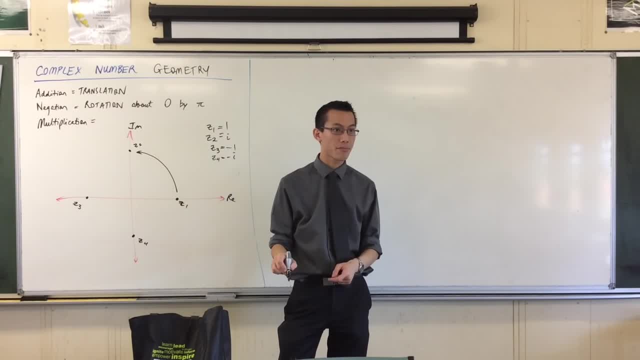 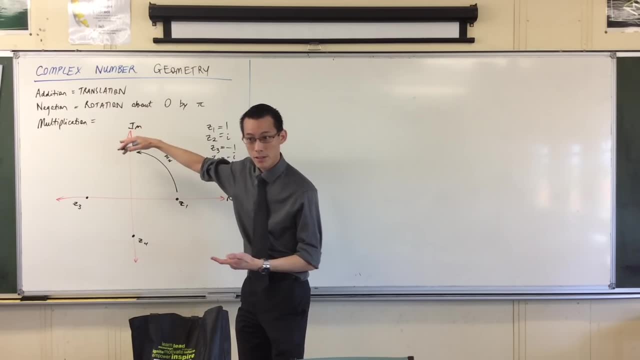 So what I've done is I've rotated this far. I've rotated in this case by pi onto radians. right, That's 90 degrees When I multiply by i. the second time I rotate: again: Another pi onto radians. 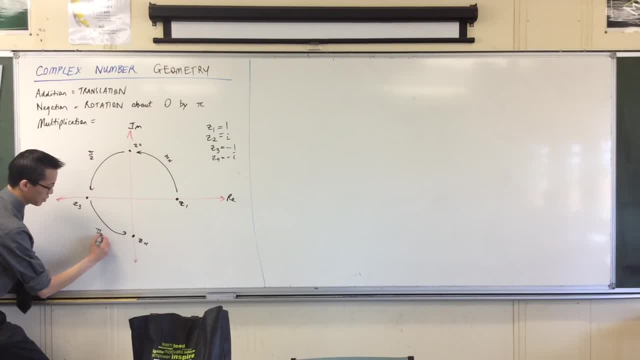 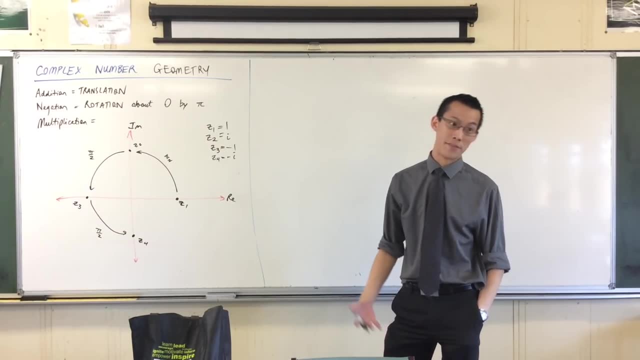 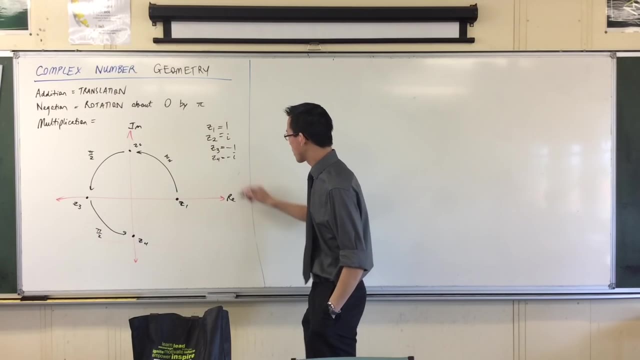 And then the last time, there's my final rotation. okay, Now you can see here: if I rotated one last time, z5, where would z5 be Back at z1. He'd be back here. and the reason why is because, multiplying by i four times, 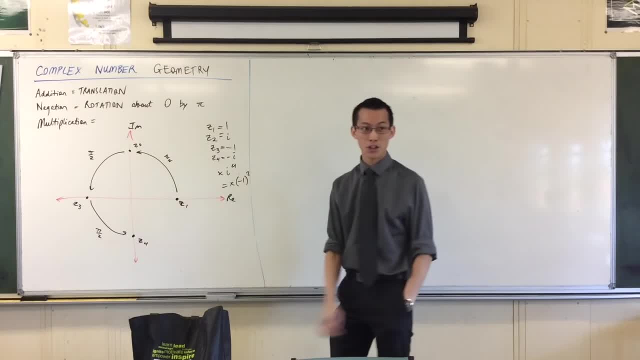 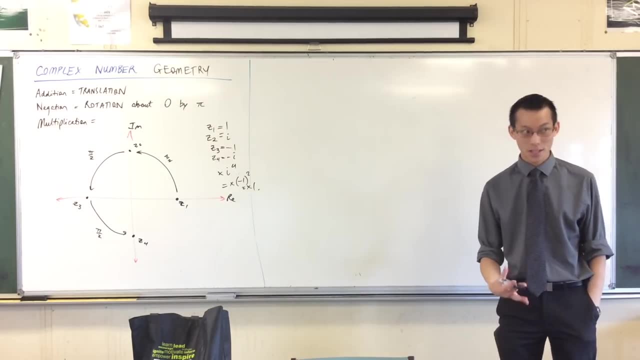 is the same as multiplying by negative 1 two times, which is the same as multiplying by 1. And it lands you back where you started. okay, What's something you can do four times and you end up back where you began.